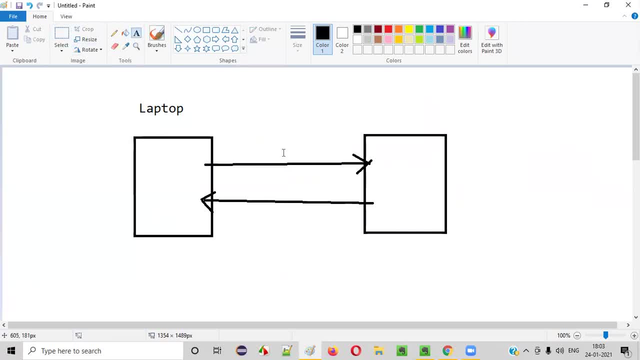 uh, I provide this. uh in place of arun. I provide some untrusted data. okay, in place of arun. if I send some untrusted data, this untrusted data, and as a response, also it sends this untrusted data, what will happen? it is a problem, right? untrusted data should not be sent in the request and response. okay, this? 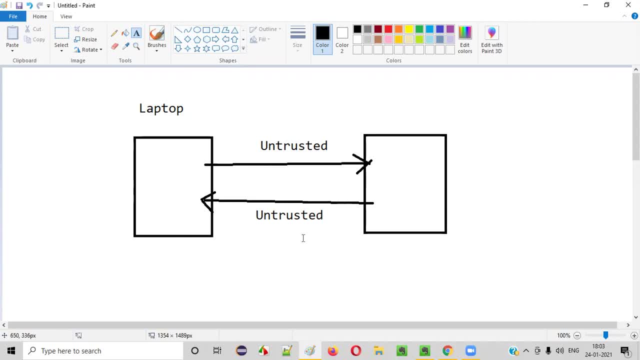 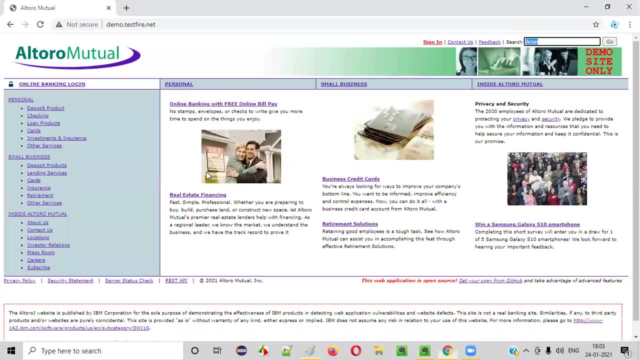 communication should not happen over the untrusted data. let me show you one such example, where client will send the untrusted data to the server and server will process this untrusted data and send it back to the client. let me show you so here, instead of giving something like: arun guys, i'm 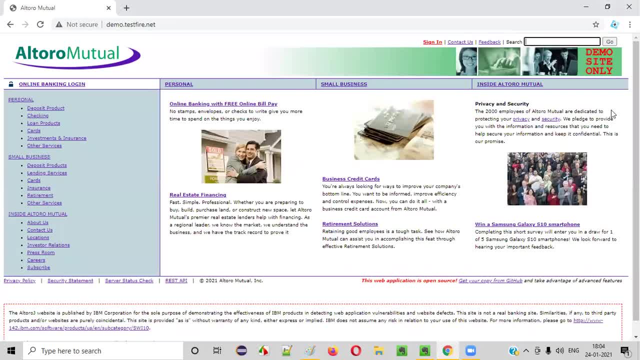 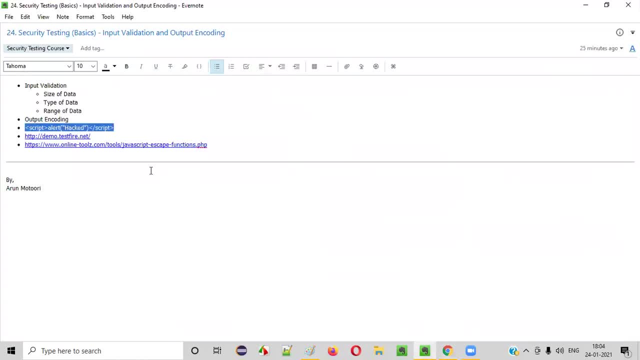 going to give this kind of thing. i'm going to run some javascript code. okay, the application should not allow you to enter the javascript code and you know. you know it should not run, actually, this javascript code. if i enter here and click on the go, this particular code should not run, guys. 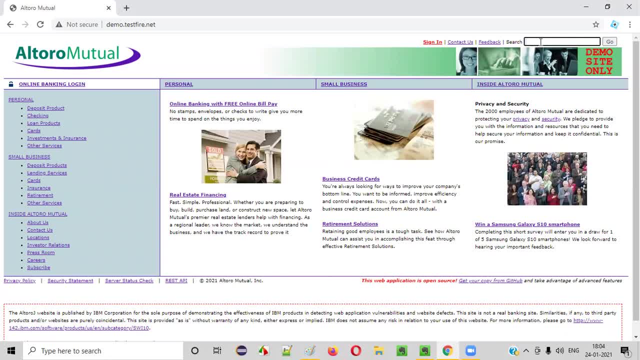 there is a problem in this application, if that happens, right, so let me write the code. i'll say script, slash, script. in between the script, i'll say alert. okay, this is a javascript sample. javascript javascript code. guys, i am trying to enter into this instead of providing some proper data in 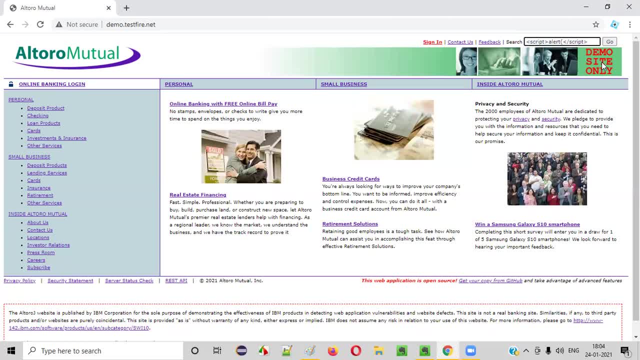 the search box field, i am entering some untrusted data, like this javascript code: here i will write something like hacked- okay, here i will write something like hacked. so and now, here this is an input field. here i am giving some javascript code and when i click on this go button, okay. 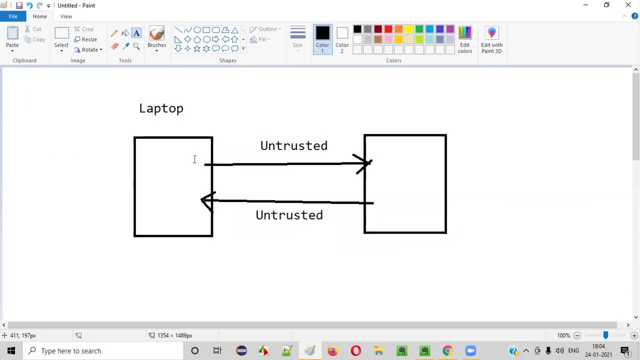 so that means the moment i click on the go button. if this particular application accepts this untrusted data, okay, then this untrusted data will go to the server server will process this particular javascript code and will respond here and whatever the browser does. right, that is a. 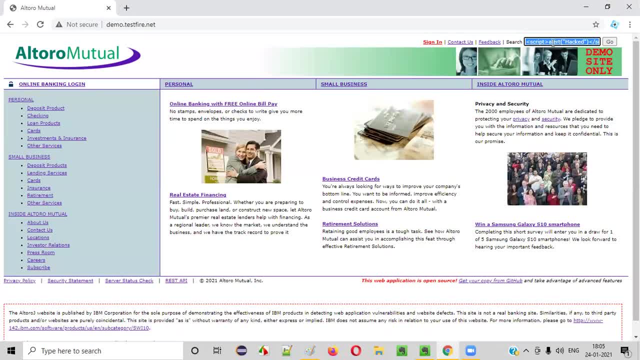 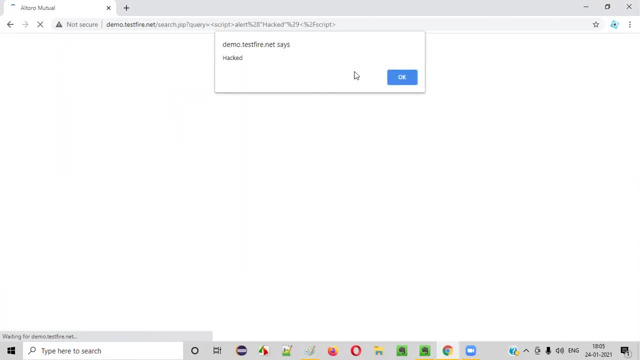 response from the server, guys. so if it is getting javascript code is getting executed or not, we can find it out. so when you click on go here, you see what's happening, guys. you are suddenly getting this alert message on your web page saying: you are suddenly getting this alert message on your web page saying: 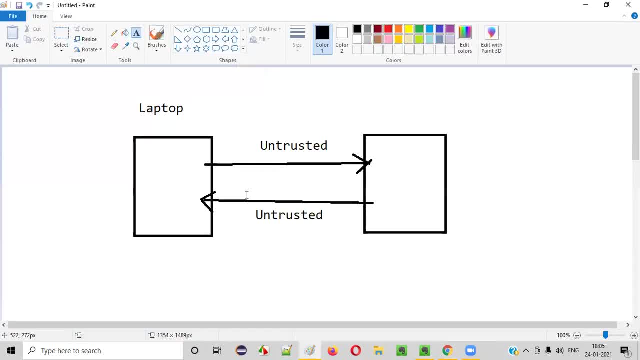 hacked. okay, so this is not good, right? this is not good. that means client is able to send the untrusted data to the server and server is able to process this untrusted data and send back or respond back this untrusted data. so this untrusted data is getting executed on your browser. so this 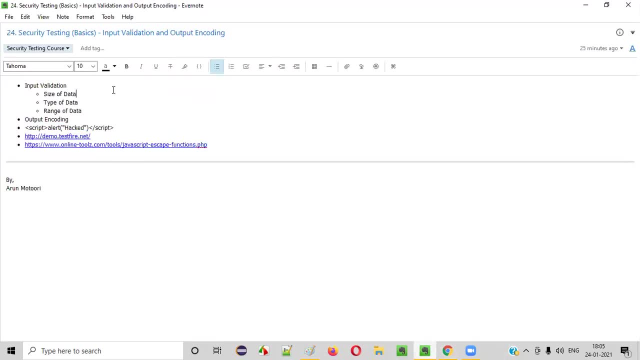 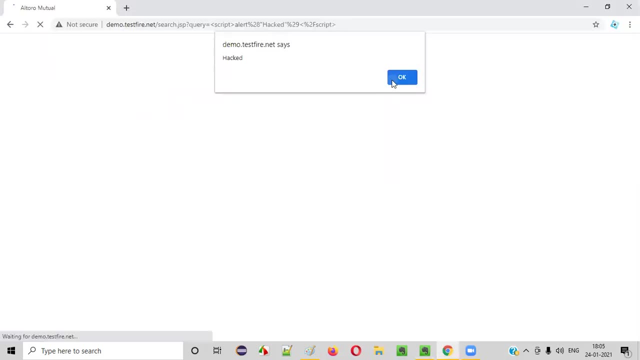 is what is happening, guys? this is all happening because of these two problems. okay, you have not put the measures for input validation and output encoding in this particular website. this particular website does not have the measures for input validation and output encoding in this particular website does not have the measure for input validation and output encoding in this particular. 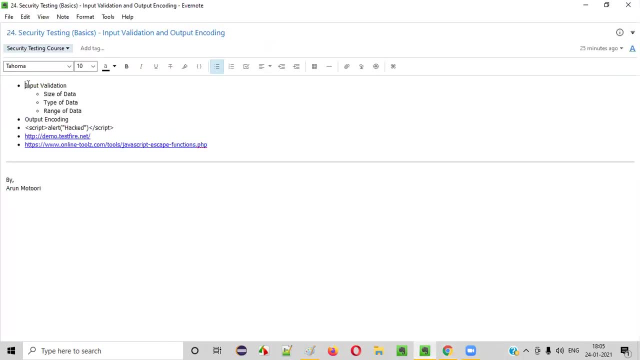 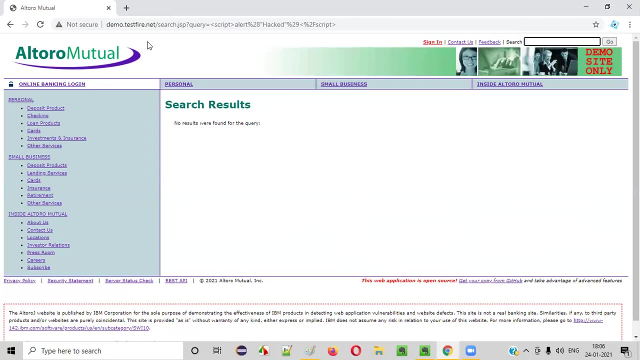 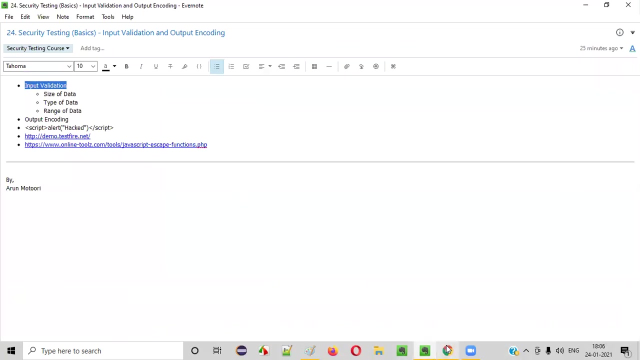 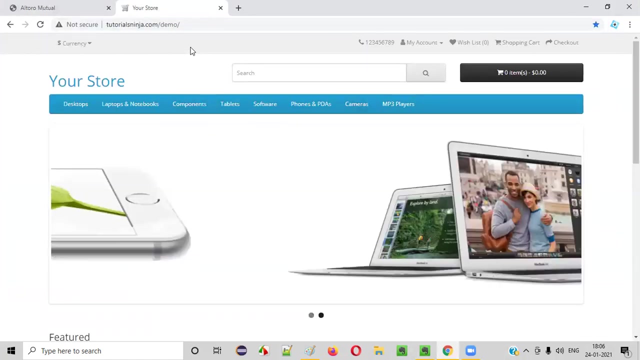 website. this particular runs. this has a history, so it does not have a proper input validation and output encoding. so what exactly are this input validation and output encoding? how they prevent this kind of stuff in this kind of websites? let me explain. so, first of all, what is input validation? anything, guys, you, it is a very 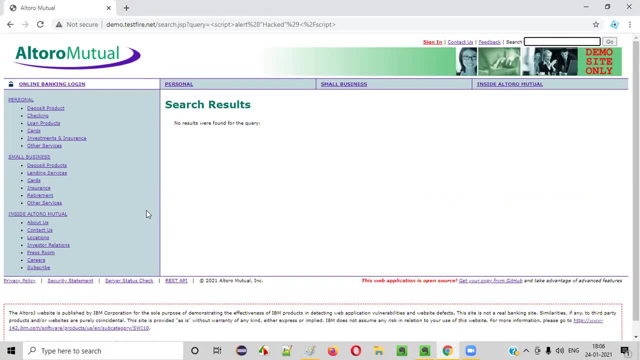 basic concept, guys. input validation is a very basic concept. if i take you to one of the website here of thing like this website, demotestifynet is a open website for performing the security testing guys. okay, so in one of the previous session i explained: right, uh, you should not be performing. 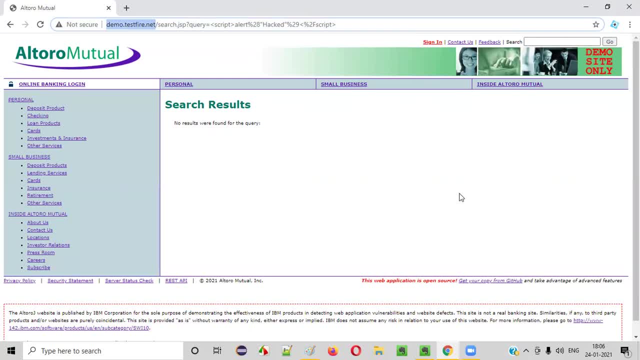 security testing on some unauthorized applications. okay, if you have the permissions for doing the secure testing, then only you will be doing the secure testing on the applications. but if you don't have the permission, don't do it guys. you may end up in jail. so one of this. but how can i show? 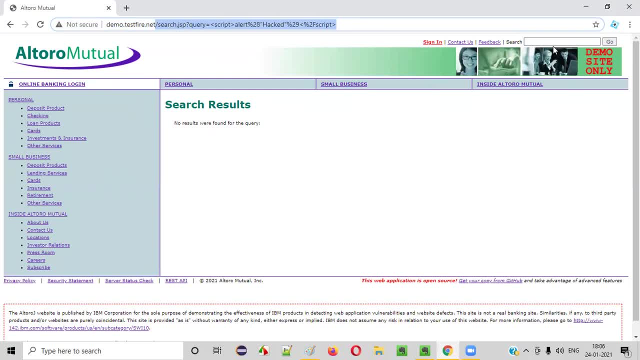 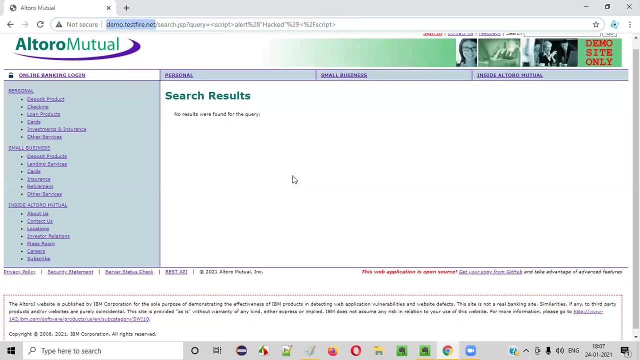 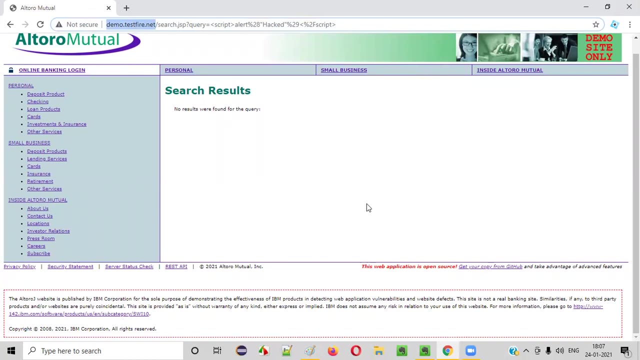 you this kind of examples like uh, exuding this javascript code, this kind of websites, because this application is open for security testing. you can perform security testing on this website. so this application is a demo site which is intended for performing the security testing. it's open for performing the security testing, so that's why i was able to demonstrate here. now let 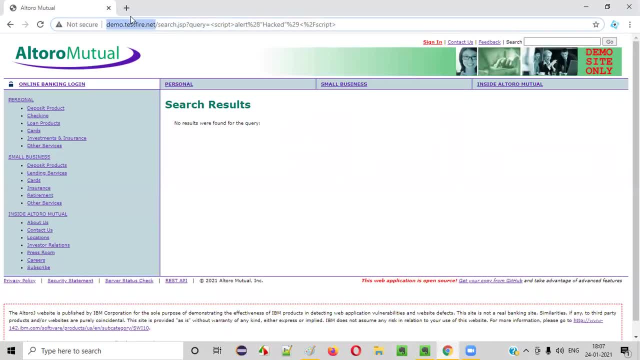 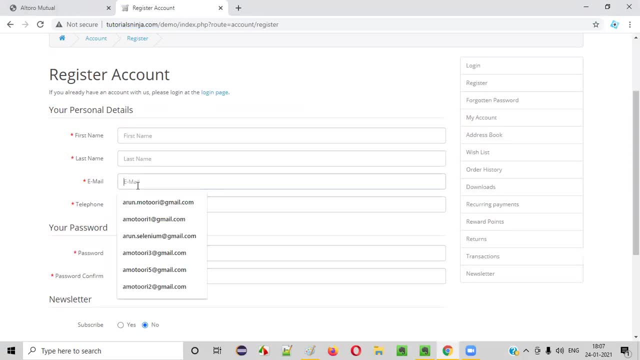 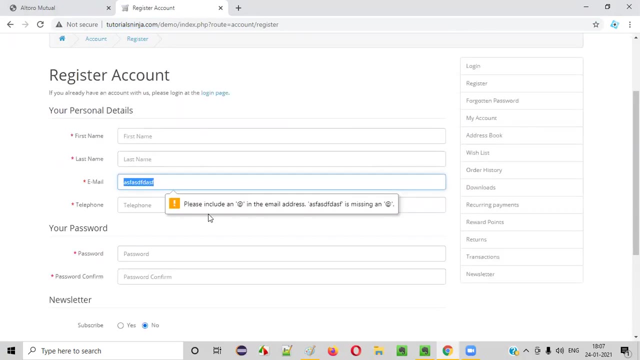 me explain about this input validation. so what is this input validation? basically, if you go to this sample website here and go to the register page, here, guys, there is a email field, right? so if i enter some non-formatted email address like this and click on the continue button, what will happen? it will say: please include an at the rate. so it's. 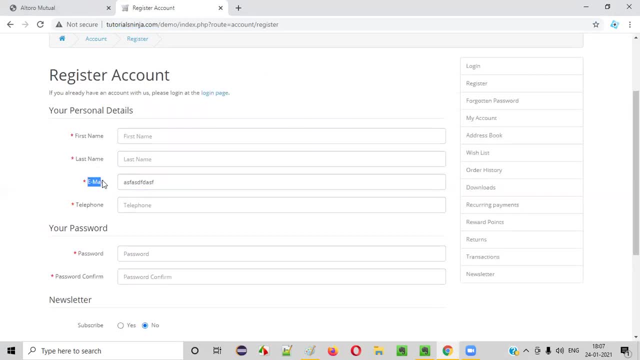 not accepting. right, there is a validation set here. but for this particular email text field, okay, if i give some proper formatted email address, only it is taking. if i give like this, it will take because something at the rate- somethingcom- is something: the valid format of the email. 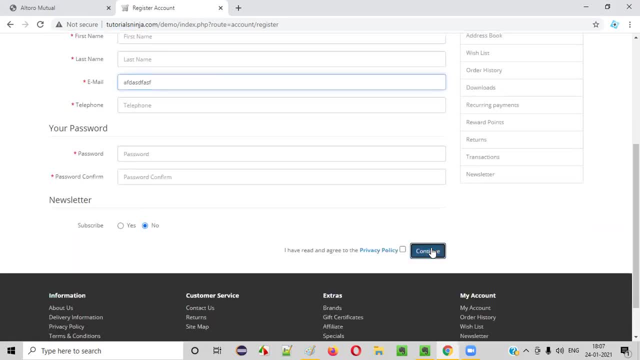 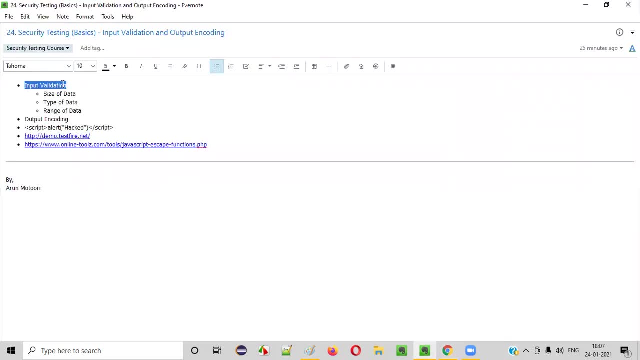 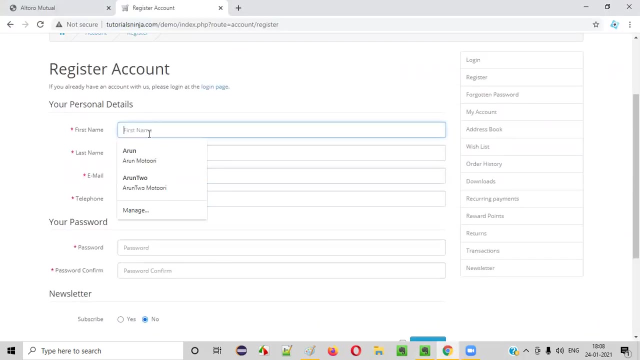 but if you give something like this, okay, some invalid form, it it's not taking. this is called as input validation. guys, here type of data matters, format of the data matters, right? so input validation can be done like this: based on the size of the data. okay, that means in a particular text field. let's say there is a particular text. 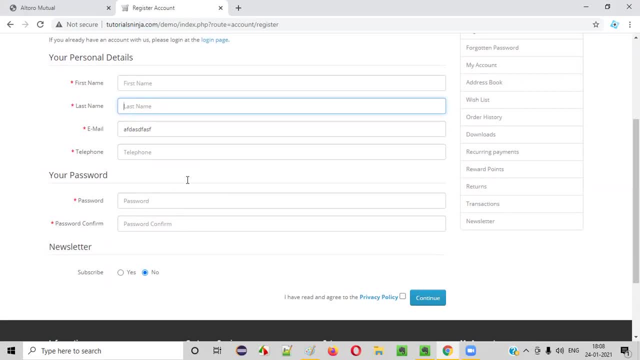 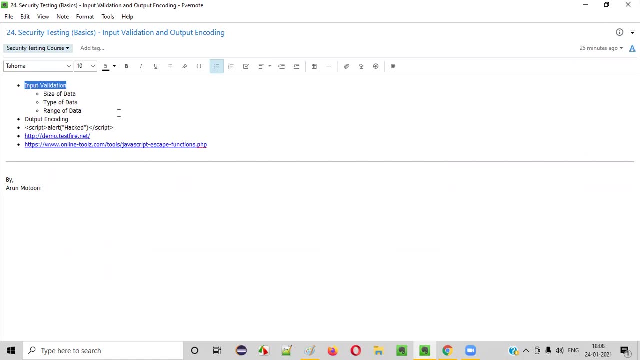 field into which you can only enter some five characters or up to 10 characters. that is size of the data. that is one type of input validation. okay, it will not accept if you enter a level 12, 13, size of the data. type of the data. so if a particular text field is a particular text field, 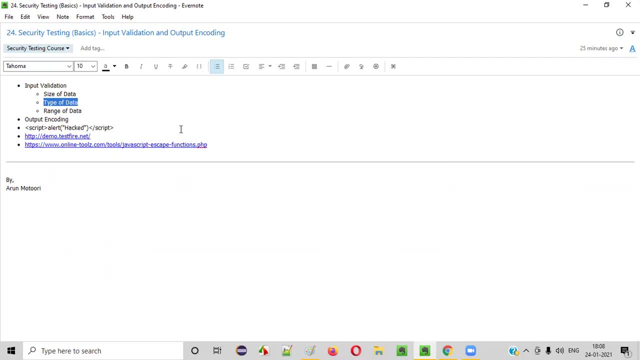 is accepting only numerical values. if you try to enter some text, then if it is. if it is not accepting, so that is based on the type of the data input. validation is done based on the type of the data there, because the input field where you are trying to enter the data is accepting only the numerical. 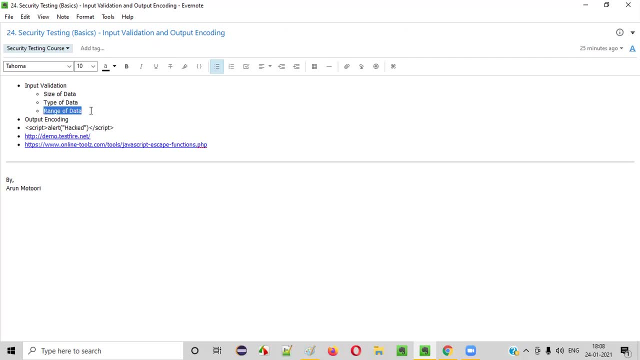 fields, not text fields. so other thing is like range of data. let's say there is a text field where you can enter the age: okay, from one to nine. okay, only in the range of one to nine you can enter the rate, apart from one to nine. if you try to enter anything like, uh, 12 or eight, 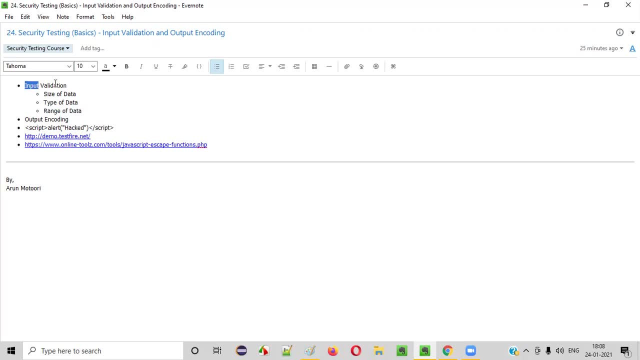 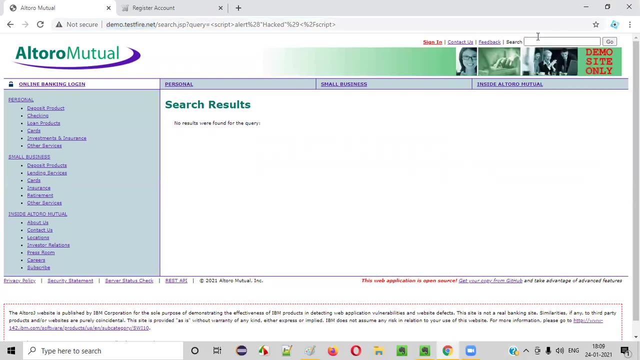 bc or whatever it is, it will not accept. so that kind of input validations are generally set for this kind of text fields. guys, okay, this kind of text fields will have. so here such box field is there. there is no input validation set for this. that's why i am able to even enter my javascript. 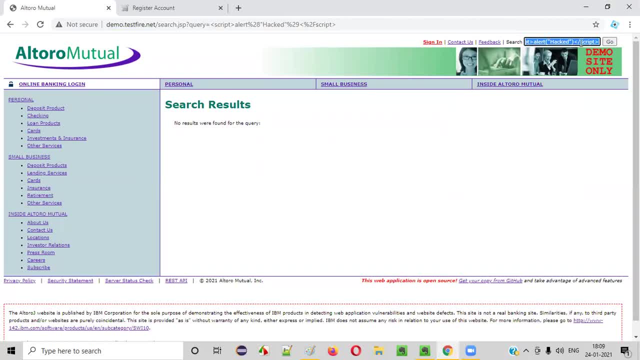 here. okay, i am able to uh process the javascript here. this particular javascript is being sent to the server of this particular application because this text field, this search text field, doesn't have any input validation set. okay, if this particular search field has some input validation set, right, like, uh, this: less than symbols. greater than symbols are not accepted. okay, or these double. 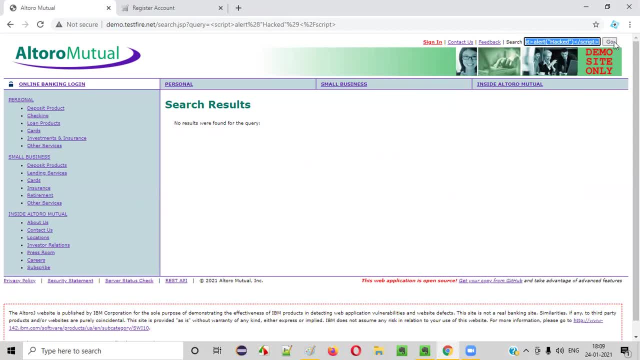 quotes are not accepted like this, then, guys, this would not have happened. if you click on go here. here you should have got the message saying that uh, enter proper data, kind of thing. okay, here you would have already got some message like: uh, enter some proper data. but here, since there is, 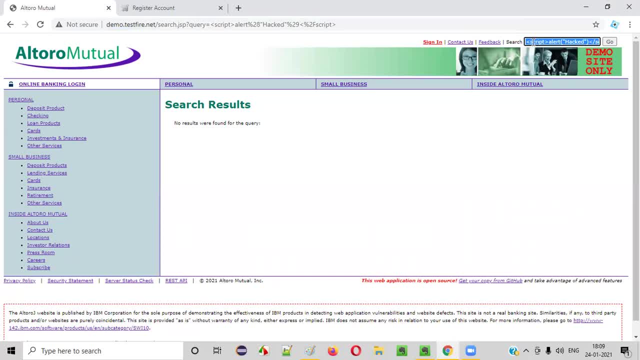 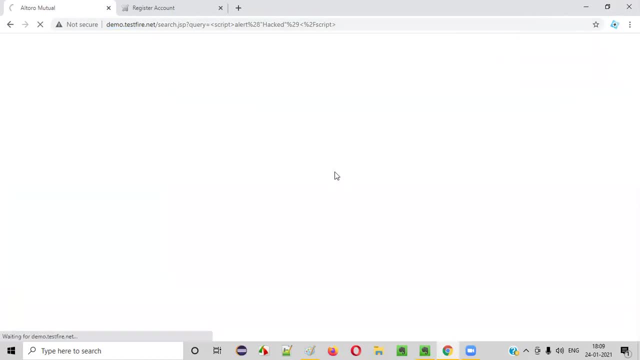 no input validation set for this particular application, this javascript code. okay, hacker will do the same thing as you will try to enter this kind of javascript code and click on the go button. fine, you see the server is processing and also it's getting executed, guys. so why it is getting? 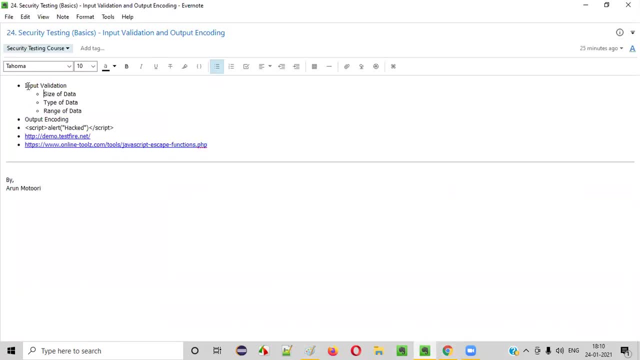 executed because of not only this input validation, guys. input validation is allowing some untrusted data to uh to be sent to the server, right, if the input validation is properly set. what will happen, guys? if the input validation is properly set, this untrusted data will not reach the server. 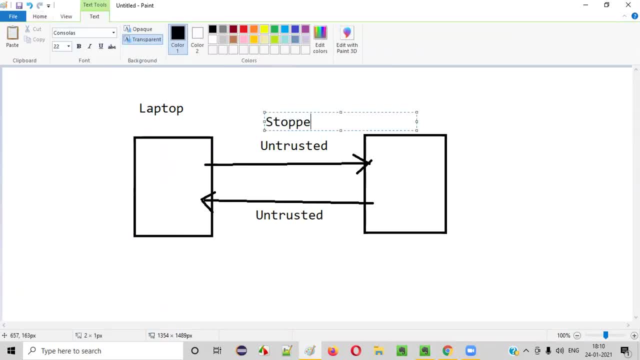 right, untrusted data will be stopped from reaching the server. if input validation is properly set, okay, untrusted data will be stopped from reaching the server. but that is not there. hence untrusted data is going to the server. now, let's say, input validation is not there, but, uh, this untrusted data went to the server. that's fine. 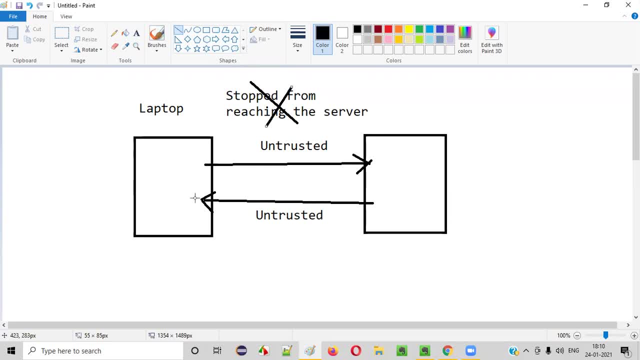 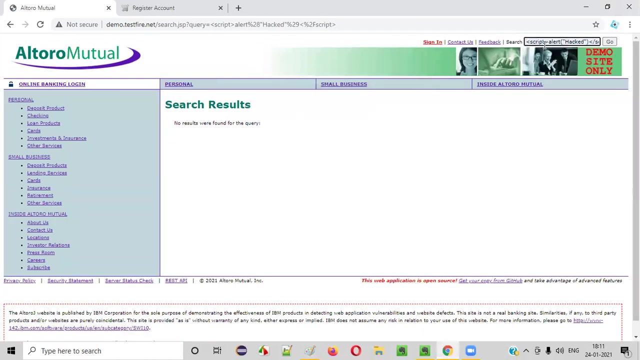 now server is processing this untrusted data and sending the same untrusted data to the application that is your client. it's another problem, guys. okay, this is another problem here. server what it should do is it should perform output encoding. what does it mean? what is output encoding? that means server is receiving this untrusted data like this. 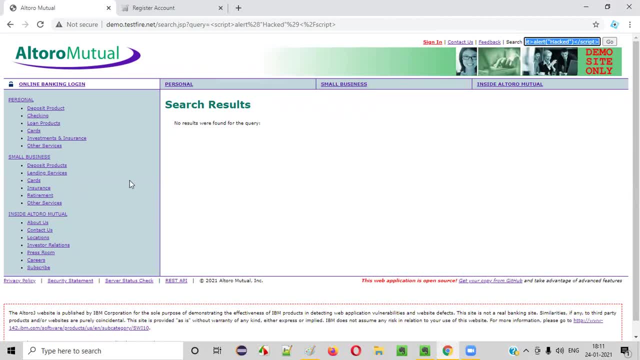 the same untrusted data is being processed by server and it's being sent back to the browser as it is, and the browser is executing this javascript and displaying this. alert guys, there's a problem, okay, how to overcome this problem? to overcome this problem, okay, not to. 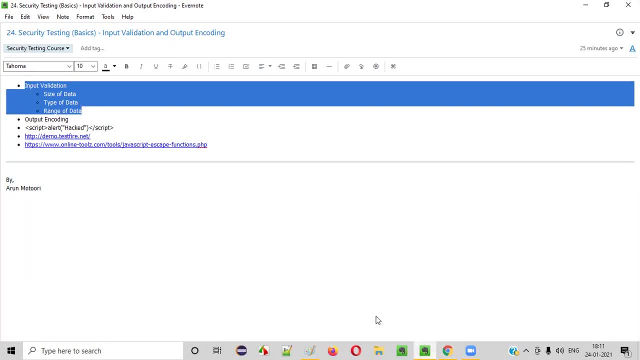 only input validation. okay, there are two problems here. input, first of all, this application doesn't have input validation and second thing is it doesn't have the output encoding. also, server doesn't actually do this output encoding. so before sending this particular same script to the back to 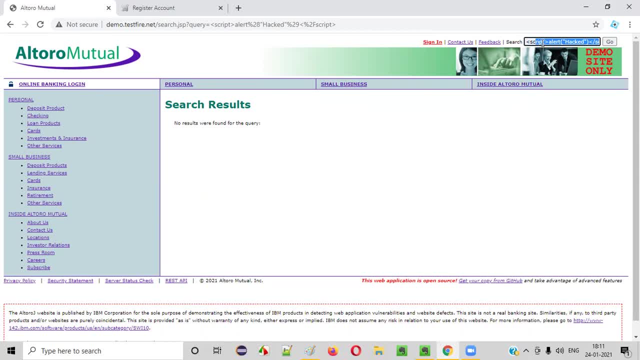 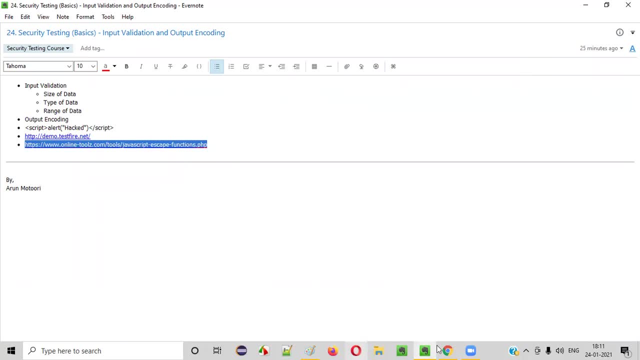 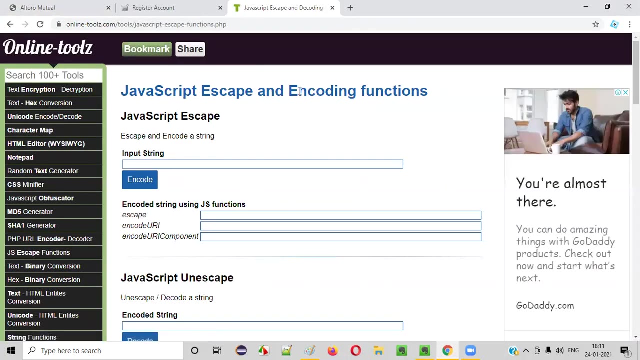 the browser and browser getting executing this particular javascript. right, this javascript can be output encoded. how to do that? let me show you something. so here is some link guys. i'll show you how it can be output encoded. okay, before coming into the output, how this particular uh javascript can be encoded so that it will not be executed or run on this particular browser like. 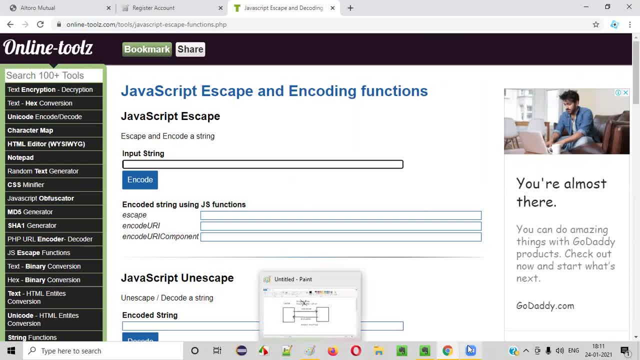 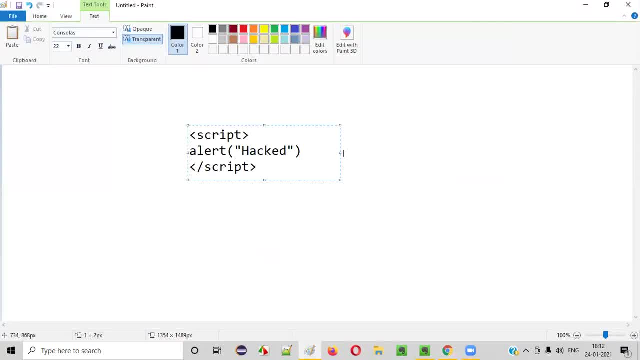 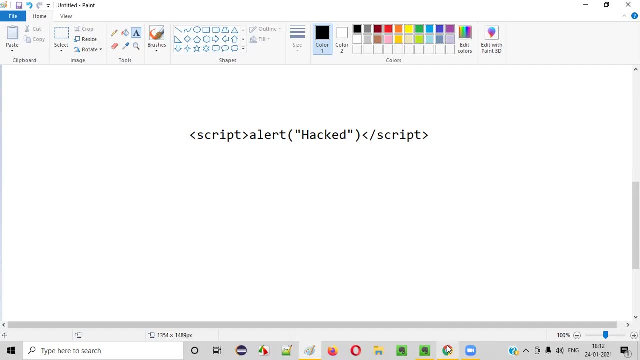 i showed you the problem that is coming here. this is the data, right? so let me take this is what is untrusted data i was explaining in this session, right? this is a untrusted data, some javascript code. so instead of the javascript code it should get an- i mean output encoded. guys, how it can get? 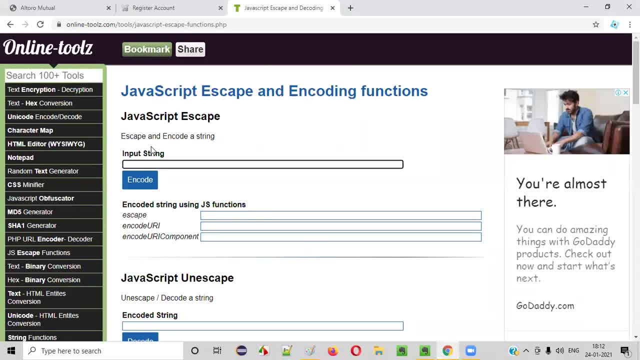 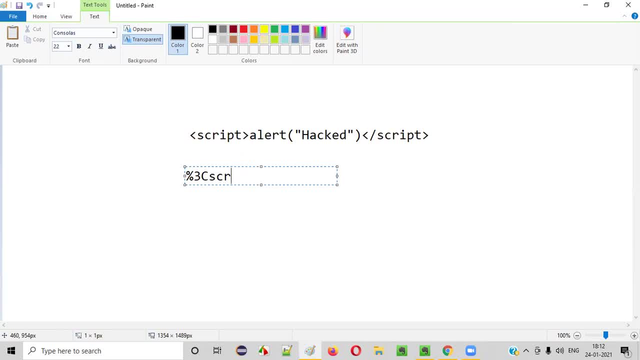 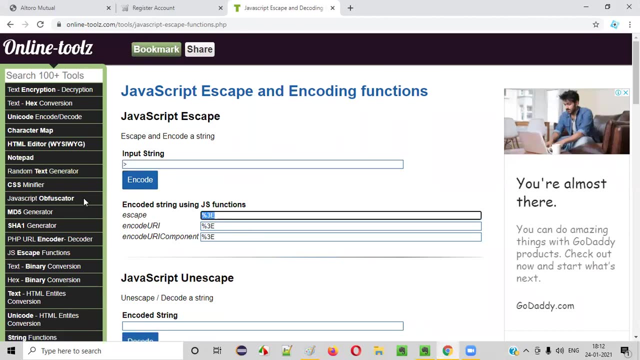 output encoded, for example the symbol less than symbol, is there right? less than symbol, so encode. you'll get this kind of text: percent lc, so percent lc, then script, script. then greater than symbol, greater than symbol: encode. so this should be converted like this. this is what is called. 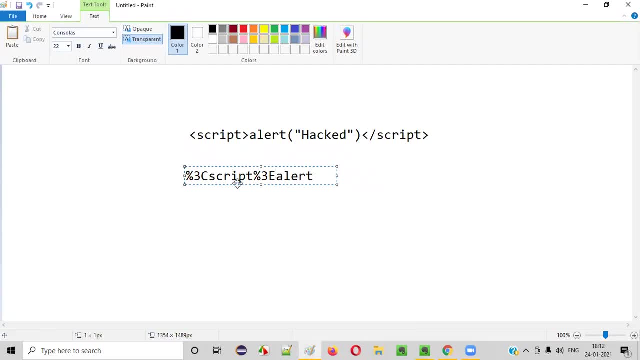 encoding guys. okay, if if the server sent this kind of encoded text back to the browser, right, browser will not execute this particular text. browser will not be able to execute this script. but if the server sent this kind of javascript code directly to the browser back, okay, in the. 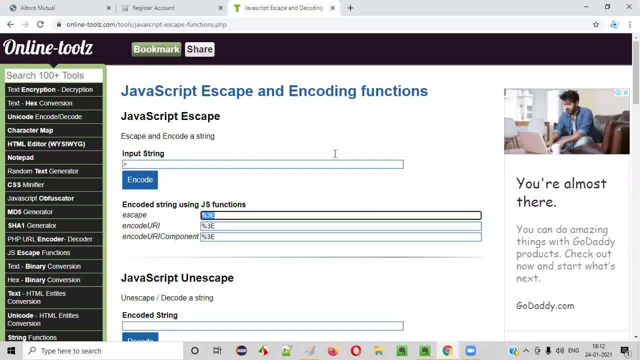 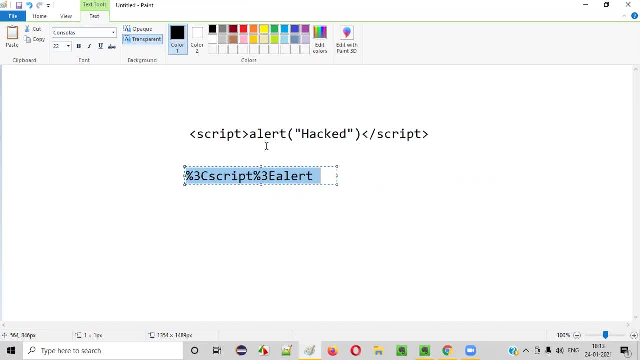 response. if the server is sending this, as it is response back to the client, then what will happen, guys? this javascript code will get executed on the browser. that's what is happening if it, if this particular javascript code, after getting processed by the server, is properly encoded like this: 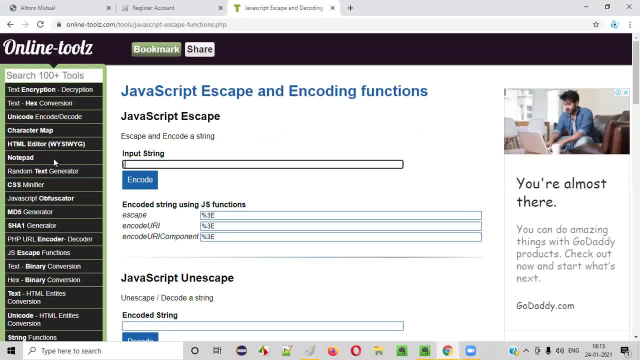 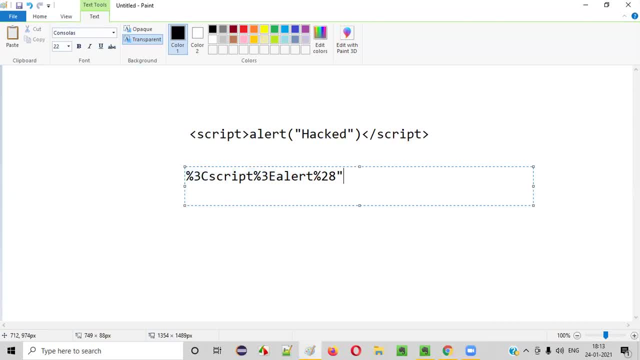 the problem will not happen, guys. okay, so here this symbol will be encoded like this: percentile to h. so this is this, what should be the kind of thing that should happen, guys, okay, so let's say hat and uh, greater than symbol. okay, so, percentile 29 and this is how it should be encoded. some characters which are not allowed. 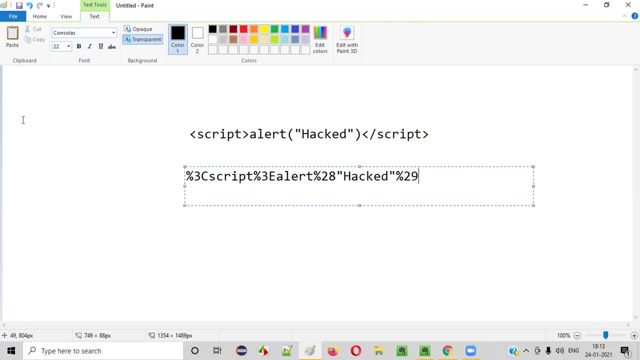 should be encoded, okay, before this particular script reaches back to the browser for execution. okay, they should be encoded and send in this particular format, so that what will happen is javascript code will not get executed. rather, what will happen, guys? rather, i'll explain you what will happen, okay, if this is, if this is converted to this kind of encoded output, encoded format before. 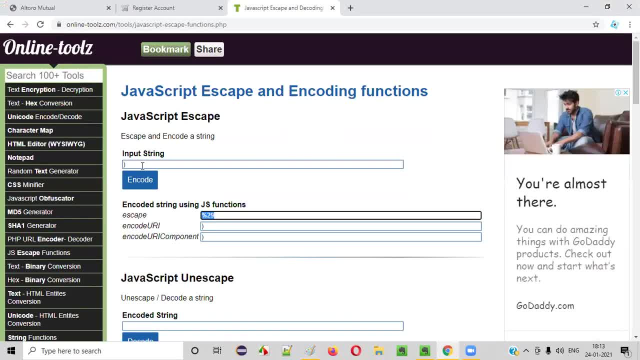 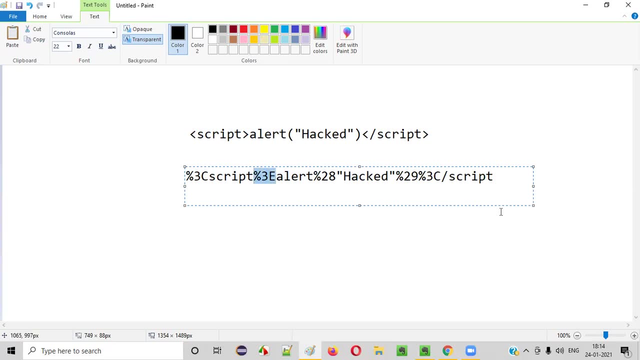 the browser. right, what will happen? let me explain. slash is there, so let me completely convert this encode. uh, let's say slash is slash, only no need to change. okay, so script and uh, this one greater than symbol, has this particular. so, instead of javascript code, if it is properly output, encoded, this particular, instead of this javascript code, this particular. 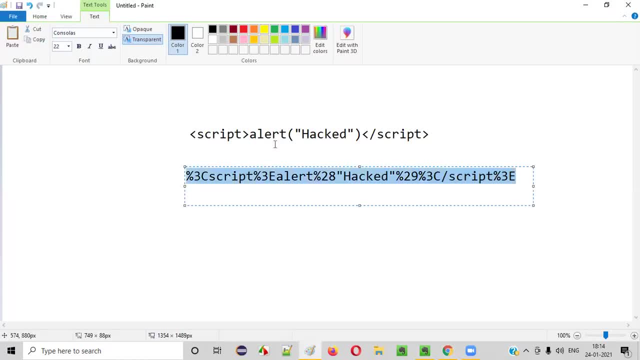 text will reach the browser right as a response server will send this particular text encoded text. if output encoding is there in this website now, browser will process this and it will convert it back. guys, okay, it will not execute, but rather it will only convert. okay, it back to the original. 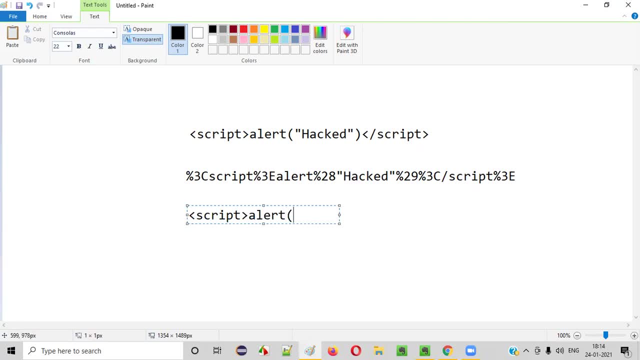 format, only this particular text will be searched. okay, instead of searching with this particular text. you see, this script is running directly, right? instead of searching this text given by the hacker. okay, the our application is running this javascript code, guys. so, rather, if the server has encoded this, 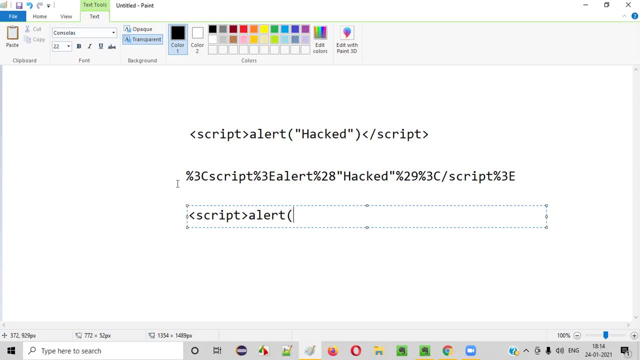 particular java script gam code to this format. browser will not be able to execute this and browser will simply decode it back to the original format and display in the search result space, but it will not be executed. hope you are able to get what will happen right. we are getting the point here what i'm explaining. 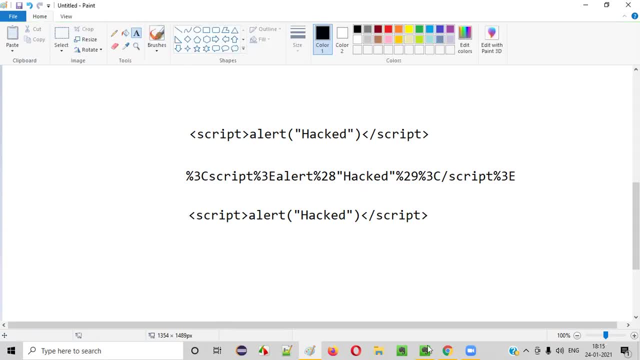 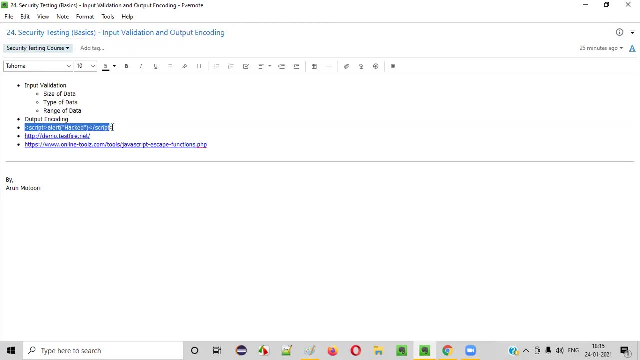 so, guys, that's the reason, guys, there's a reason we should have both this input validation and output encoding set in our websites so that hacker will not be able to run this kind of untrusted data. okay, this untrusted data should not read the server and server should not send. 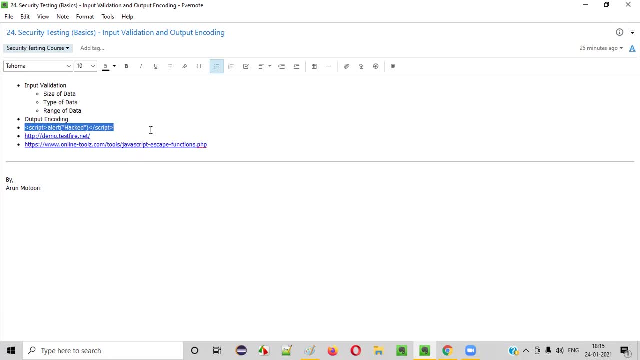 it back to the client. if it happens, what? what are the major possibilities that may happen? if this kind of thing are allowed in this, the hacker will run this kind of simple script. okay, in the initial run he will run this simple script. guys, it doesn't do anything, it just gives this kind of alert for. 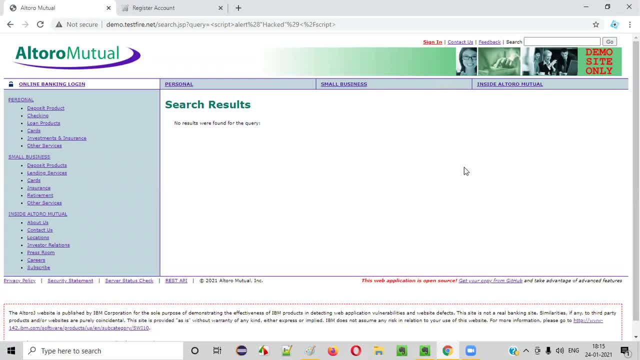 now okay. and when you say okay, everything is into the normal state. but the hacker is very clever that he will not write this kind of simple javascript code. guys, he will write some adoptions or javascript code which can steal your information in your cookies. okay, so hacker will write some.